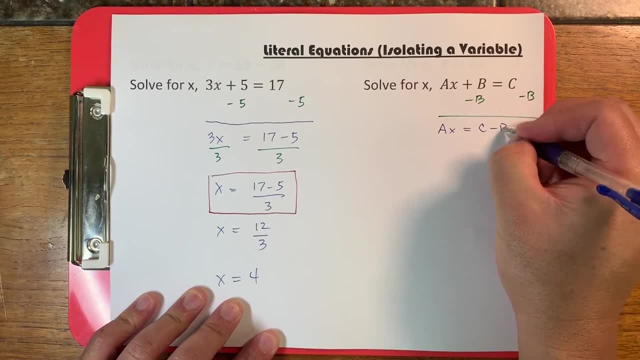 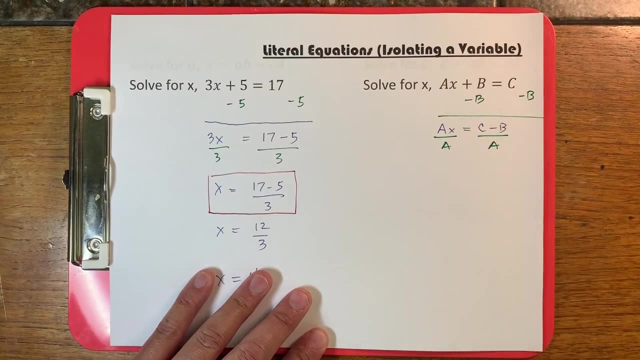 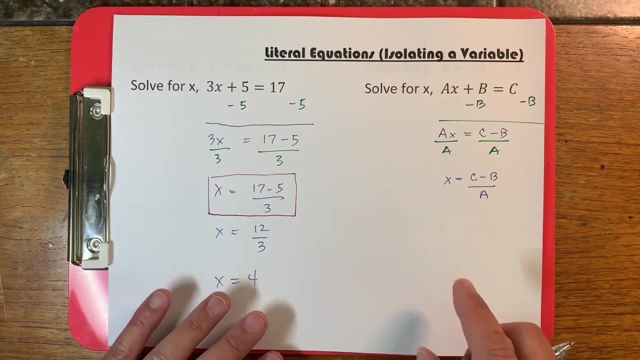 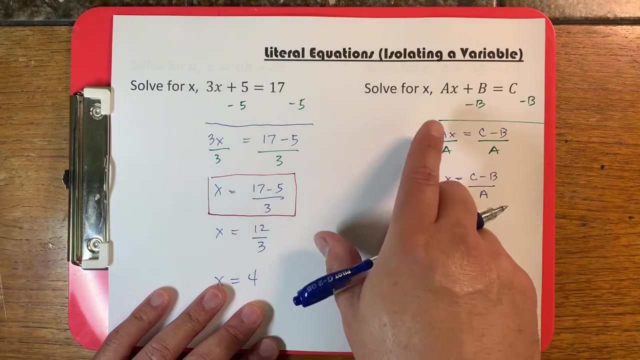 ax is equal to c minus b, and then I'm going to divide both sides by a. Now we have to stop here, because these are not numbers, these are variables and we can't actually subtract them. So if I wanted to have a formula that was based on what is x equal to? 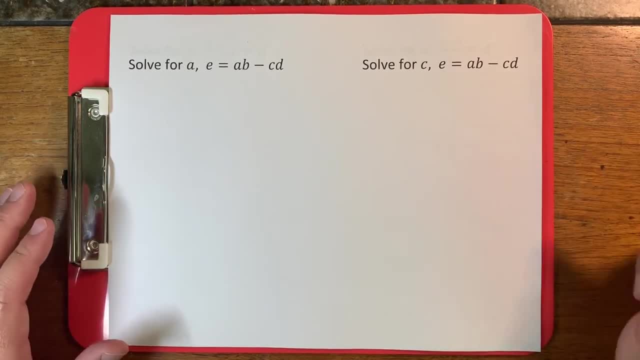 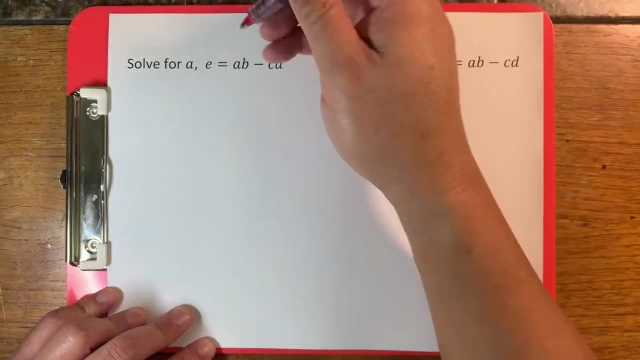 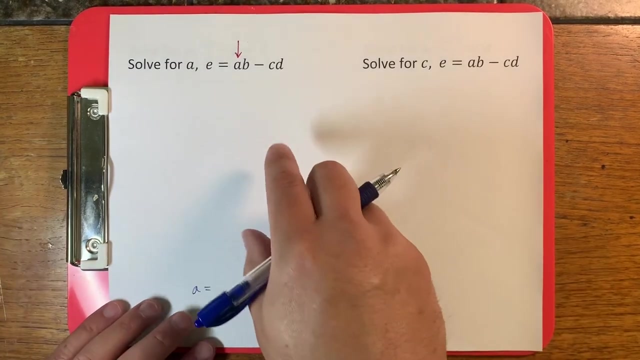 this is what it would be. Now let's do a few more of these problems. So in this problem here, what I want to do is I want to isolate the a. I want my final answer to look like a is equal to something. So the first thing I want to do is I want to get rid of the c and the d right. So 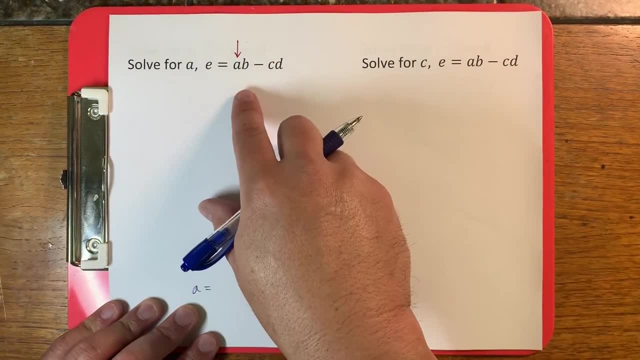 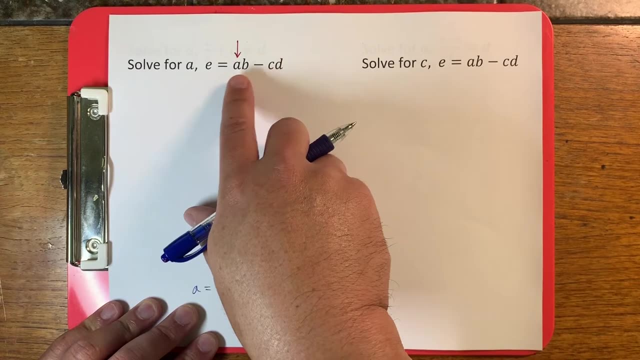 think of this as reverse PEMDAS. Whenever we do PEMDAS, we do multiplication and then subtraction. When we isolate, we do the opposite first. So in PEMDAS we do multiplication first before subtraction. When we're isolating, we do subtraction before multiplication. 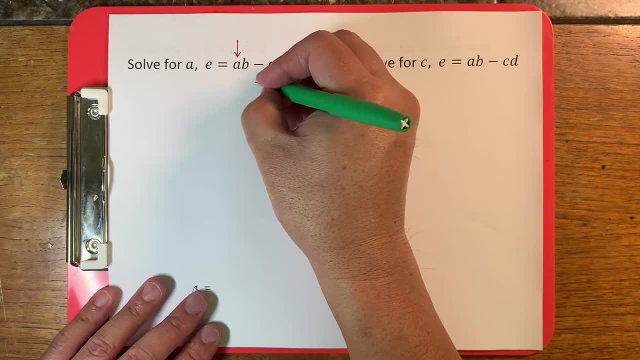 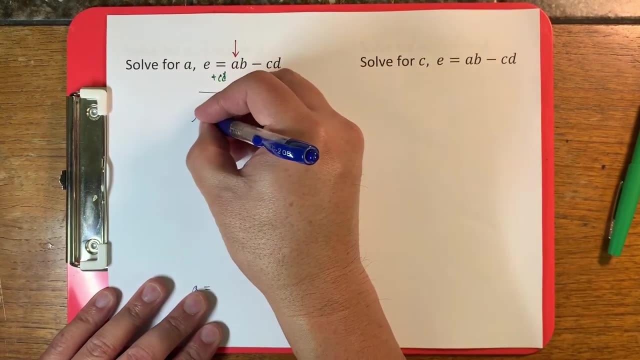 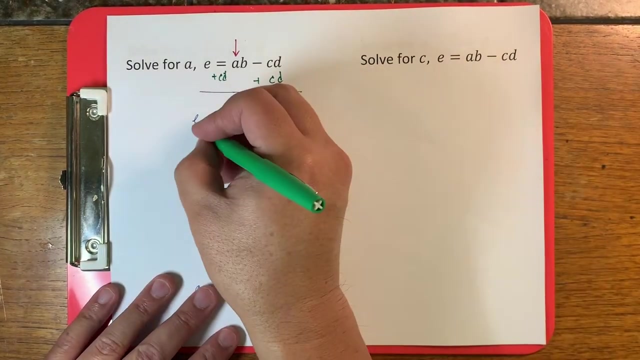 So what I want to do here is I want to get rid of the cd by adding it to both sides, And I get e plus cd is equal to a- b, and then I'm going to divide both sides by b And then I rewrite it nicely, so a is on the left side. 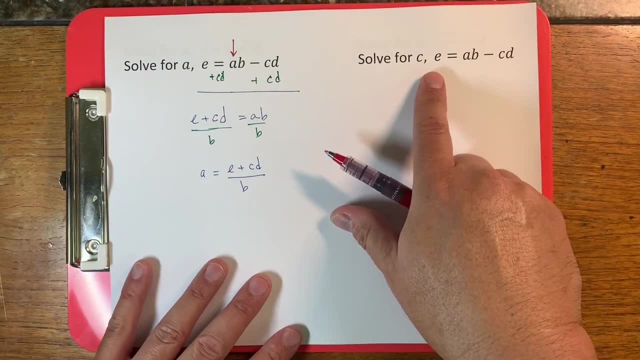 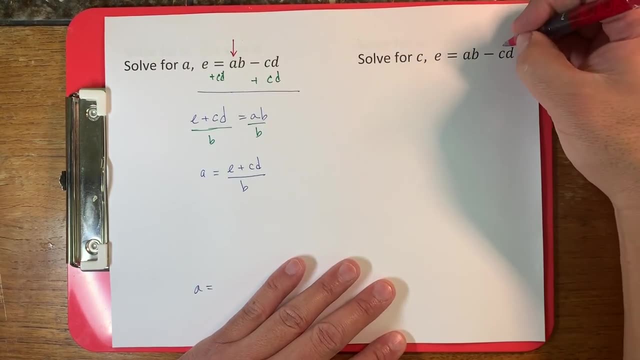 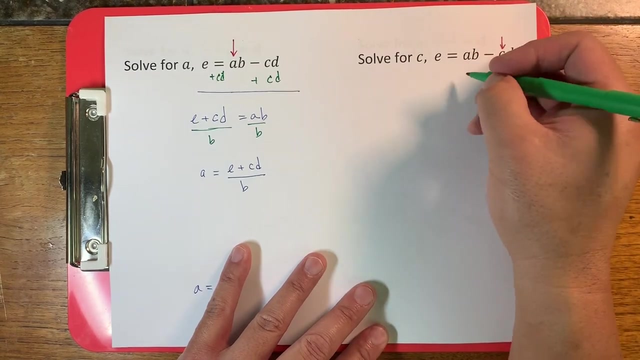 Now over here we are starting from the same equation, but what we want to do here is solve for c. So for this right here. previously we solved for a, Now what we're going to do in this one is to get rid of this. a- b first. So I'm going to subtract a- b from both sides. 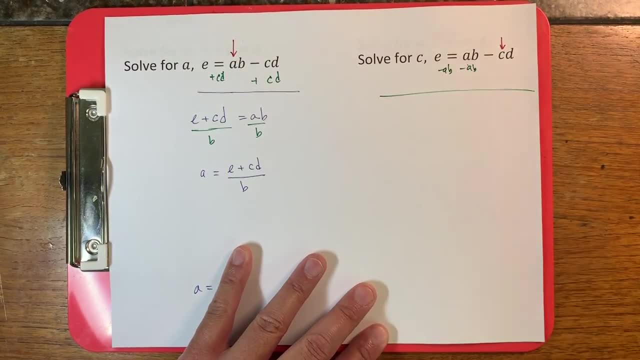 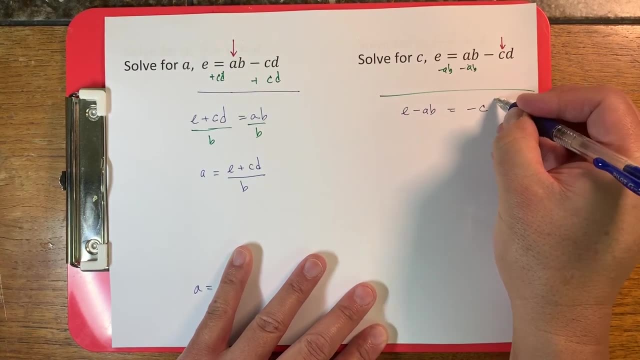 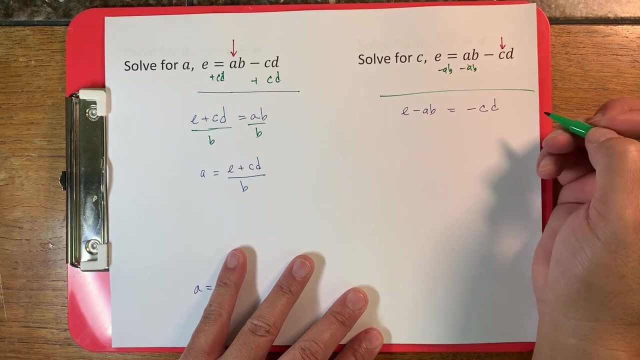 And then I get b. So here we're taking cd plus b And I get e minus b is equal to minus c d. Now what I want to do is: I want to get rid of this minus. I want to get rid of this d between the c se d is. 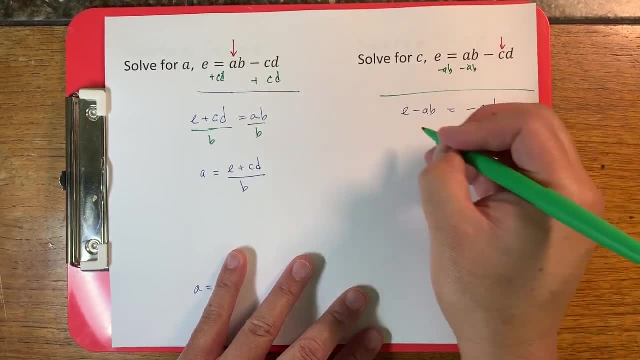 a multiplication, and the opposite of multiplication is a divide. So I'm going to divide both of these by minus d, And then I'm going to get: c is equal to e minus ab by minus cd. So again, I'm going to divide all of these. I'm going to get a c minus a b by minus c. I'm going to get c minus e, so I'm going to collect these down now. this means that I want to get rid of these minus Now. if we try to divide both sides by minus cd. 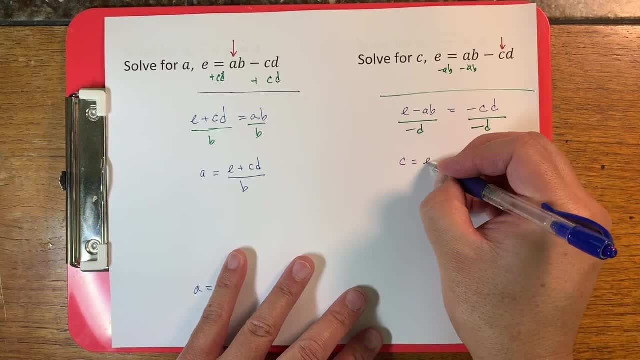 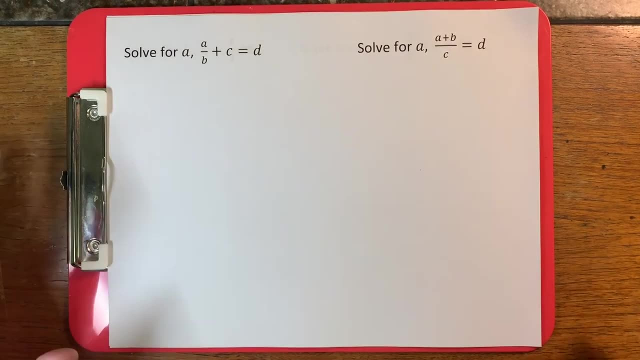 what do I want to do? Well, I'm going to use c plus c positive and c, And then I'm going to get: c is equal to e minus a, b divided by minus d. In this problem, we're going to work on getting rid of divisions. 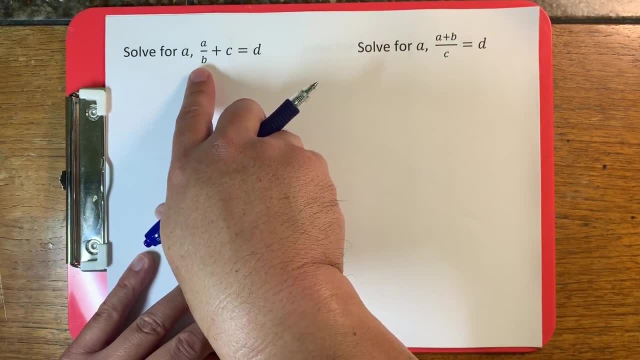 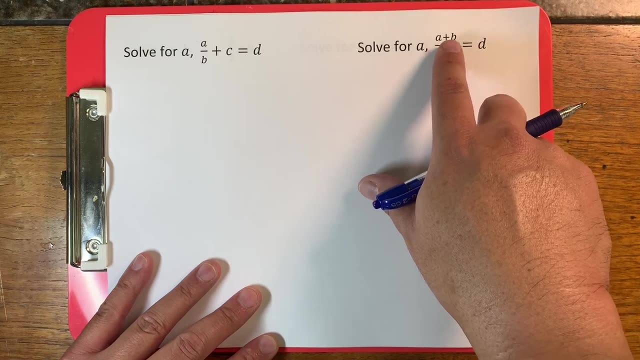 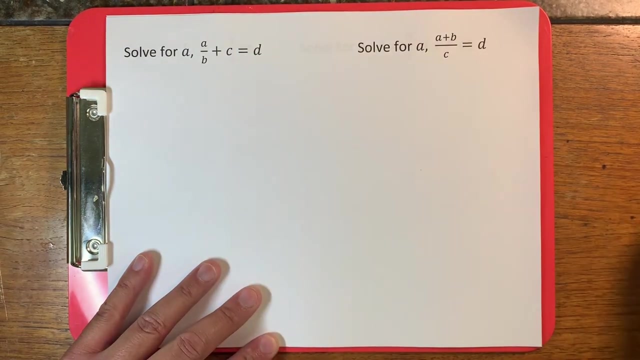 Now over here, you see the division is just connected with the a and the b. over here And you can see, over here the division is connected. the a and b are both connected to the c Now over here, because the c is separate from the a and the b. what we're going to do is we're going to get rid of that c first. 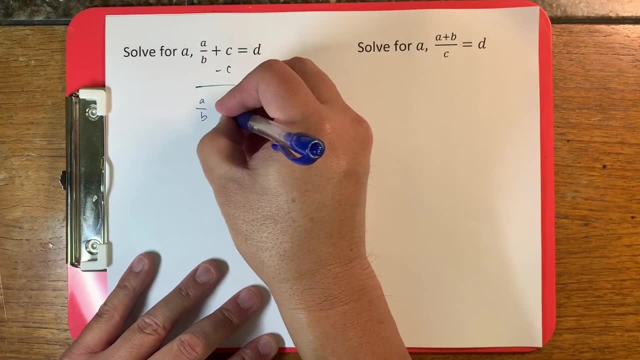 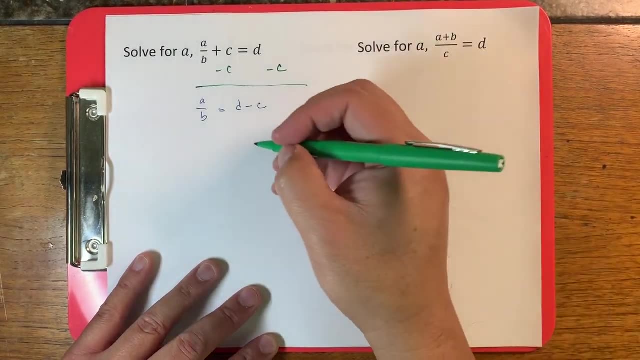 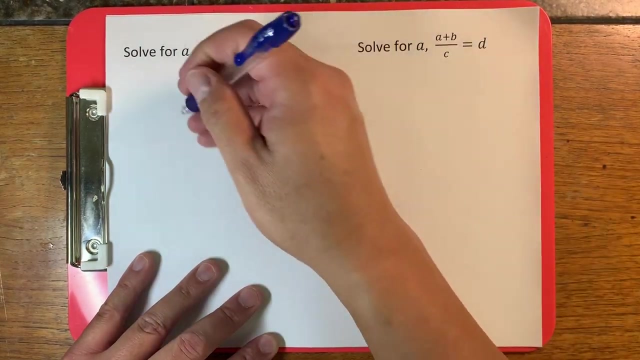 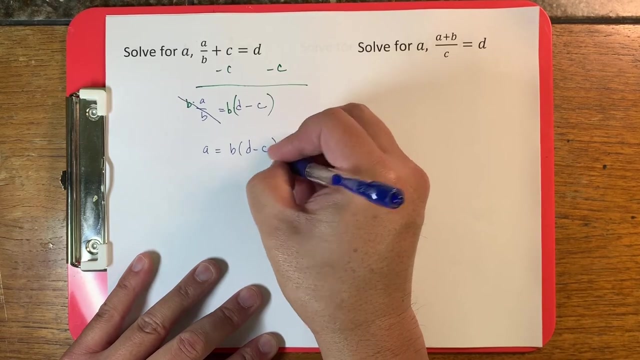 So we get a over. b is equal to d minus c. And then we're going to get rid of that b by multiplying both sides by b. So now the b's will cancel And we'll get: a is equal to b times d minus c. 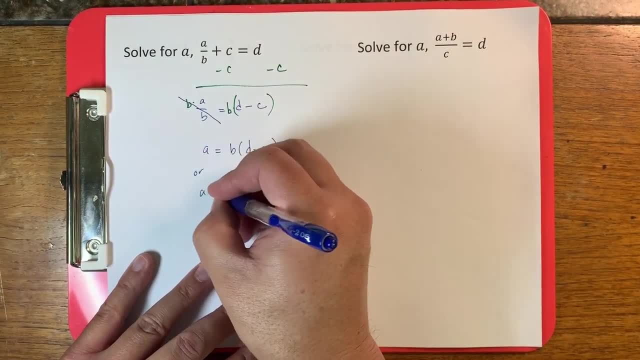 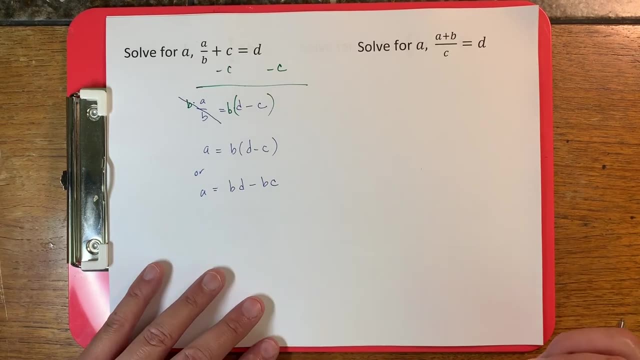 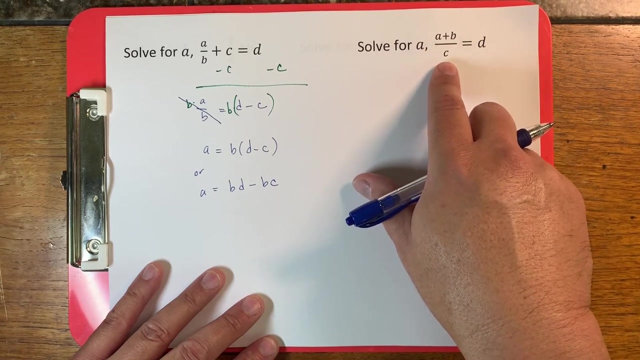 Now I'm good with that being your answer. Some people feel uncomfortable if they don't distribute it, and that's fine. also, Both of them are correct. Now, over here we can't just get rid of this b, because the a and b are tied together by this division. 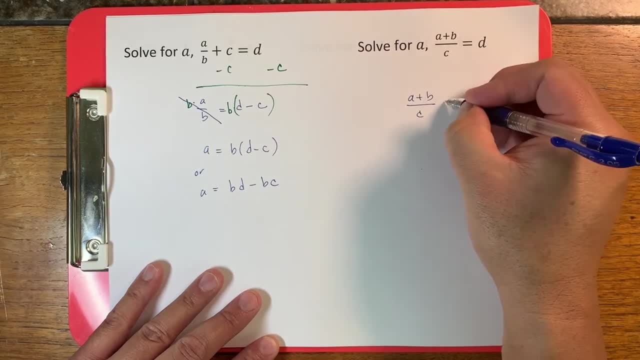 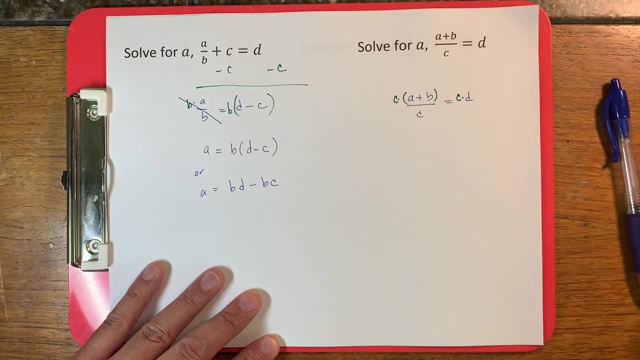 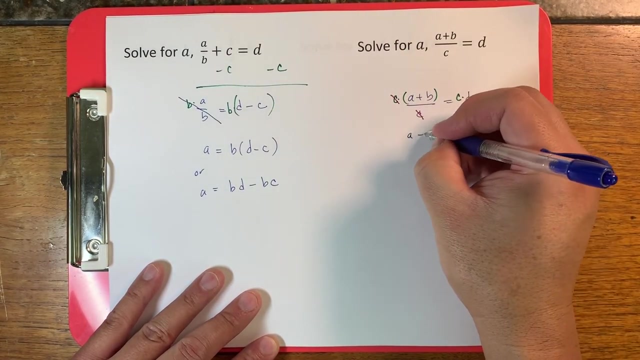 So the first thing we want to do on this side over here is get rid of that division. Okay, So I'm going to multiply both sides by c, And then what will happen is that this c and this c will cancel, And I'll get a plus b is equal to cd. 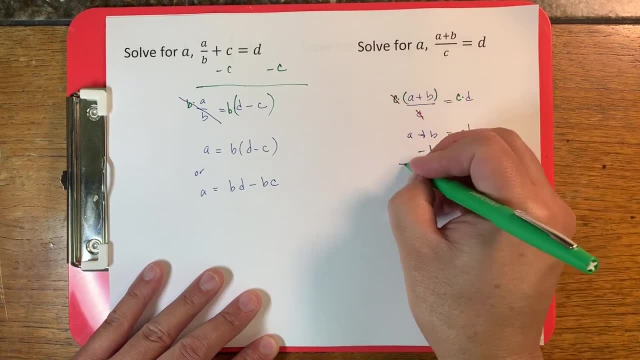 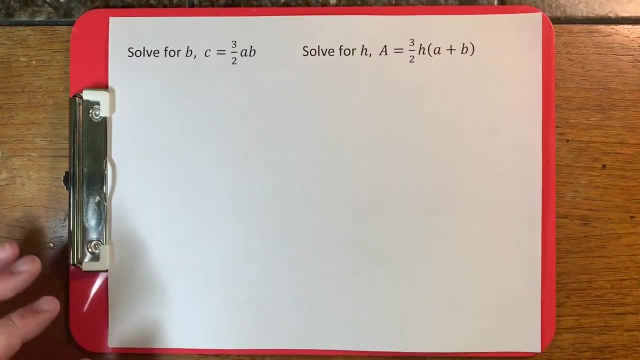 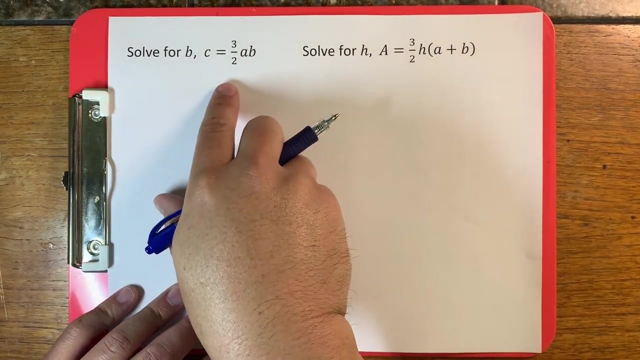 And then I'm going to subtract b from both sides And I'll get: a is equal to cd minus b. And these problems I want to show you. I want to show you the power of multiplying by a reciprocal. Let me show you what that means. 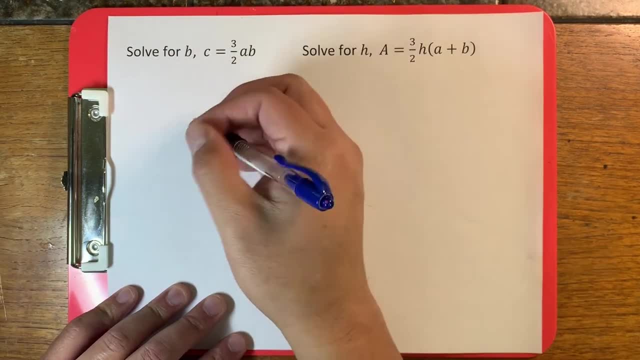 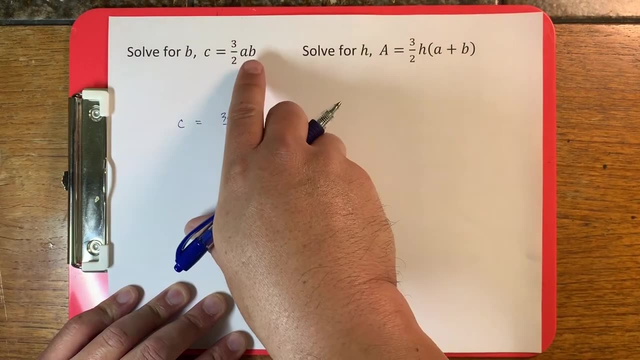 In this problem. here we want to isolate the b. Now it's easier to rewrite this as 3a over 2 times b. Now it doesn't matter whether the a's on the side or on the top. They mean exactly the same thing. 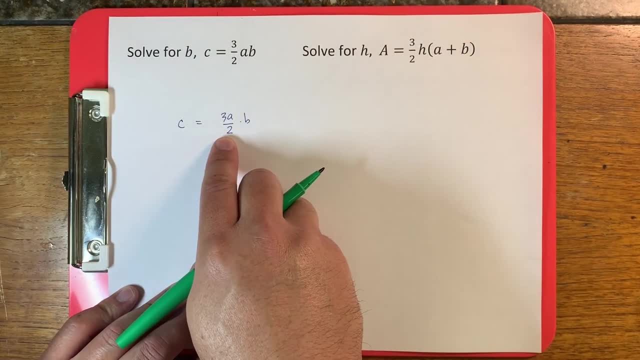 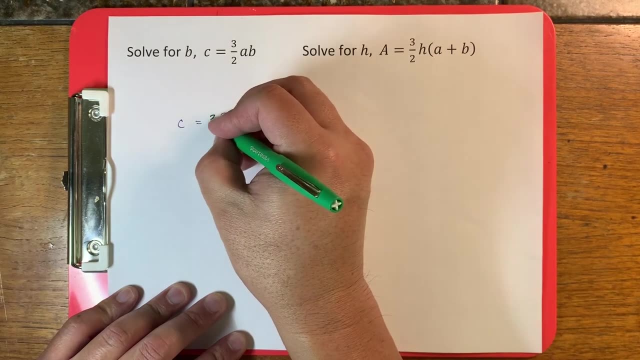 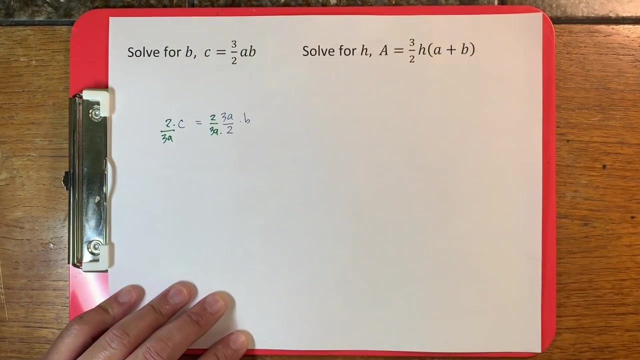 Now I want to get rid of this, And the easiest way to get rid of it is to multiply by the reciprocal, which means you flip the denominator And you do that to both sides. Now, if we look at this, that 3a and 3a cancels. 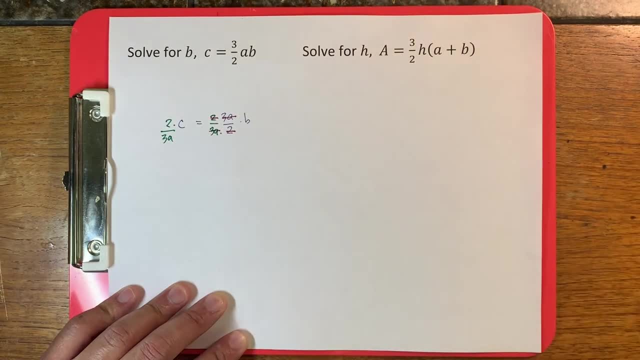 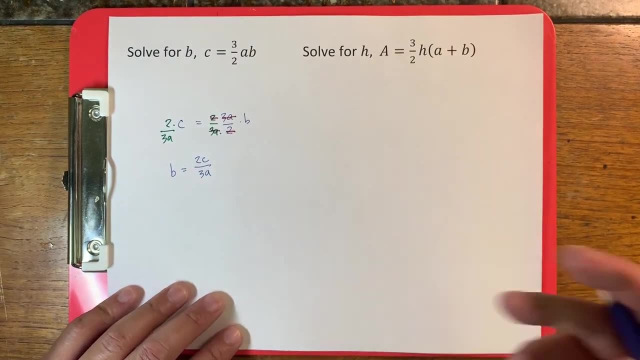 This 2 cancels with that 2. And we get the b all by itself. So now we get: b is equal to 2c divided by 3a, And then we're done. Now in this problem, we're going to attack it the same way. 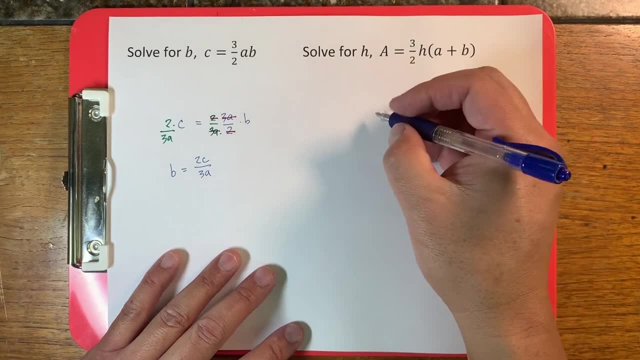 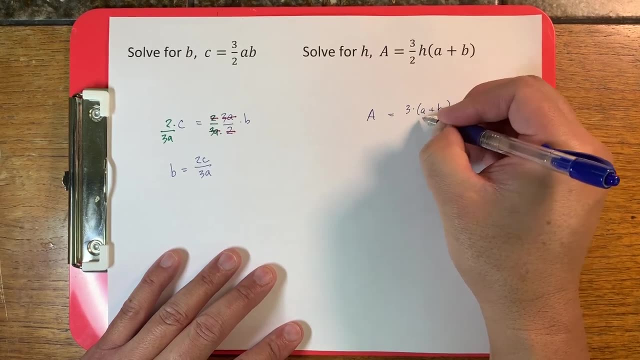 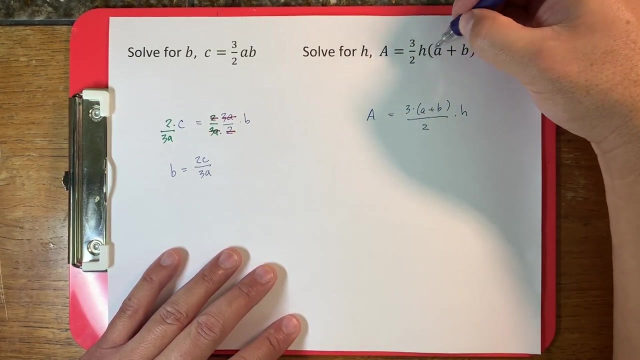 So what we want to do is isolate the h. So it's easier if I rewrite this as: 3 times a plus b, divided by 2 times h. Now notice that these are not Siamese twins. This h is not connected to the a plus b, just like it's not connected to the 3 over 2.. 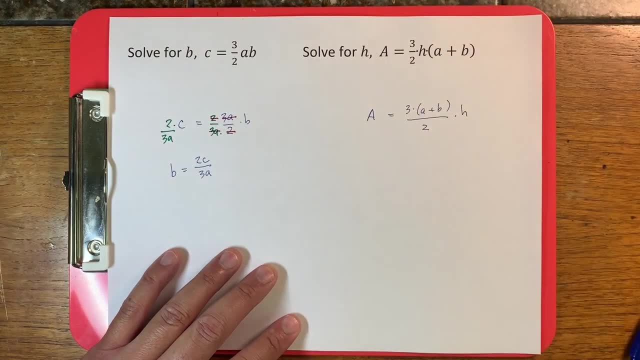 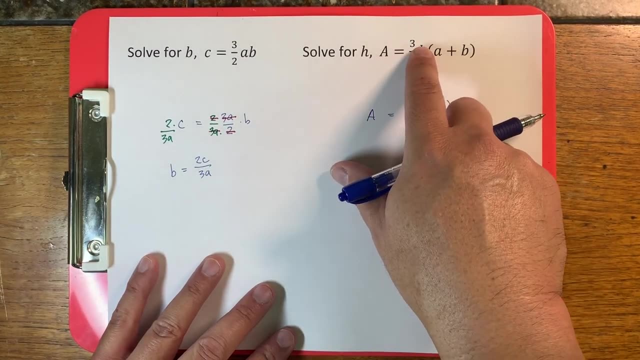 So we can put a multiplication in between them, And if things are separated by a multiplication we can move them in any order that we like. So I can move the a plus b next to the 3 over here. Now let me write this over again: 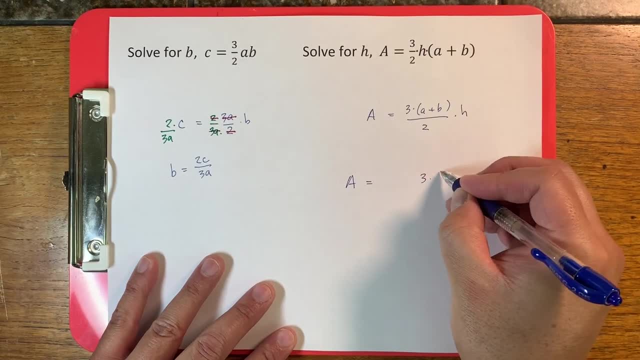 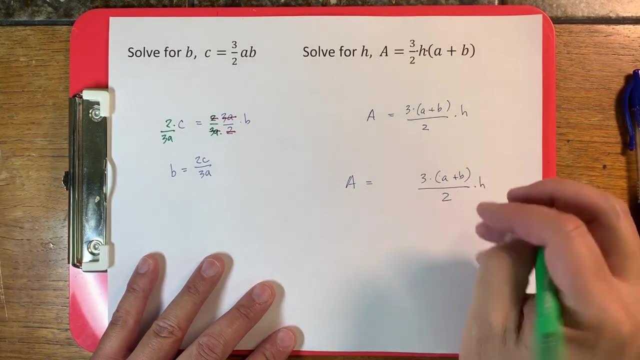 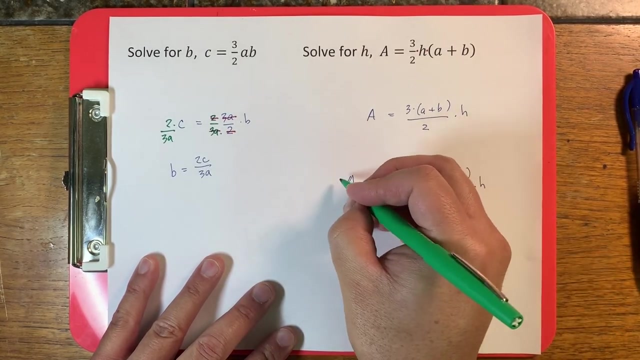 So I have a little more room to write my reciprocal. So we're going to multiply both sides by the reciprocal. We're just going to flip this right here: 2 over 3, a plus b, And we're going to do it to both sides. 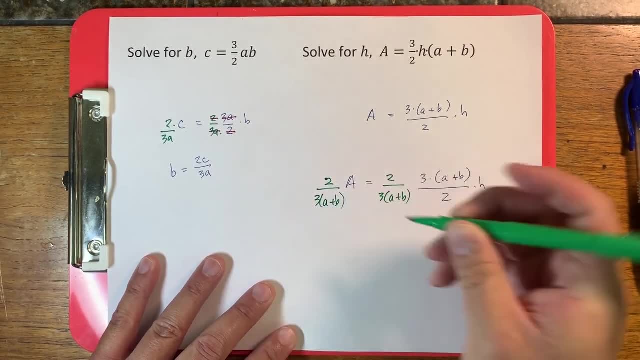 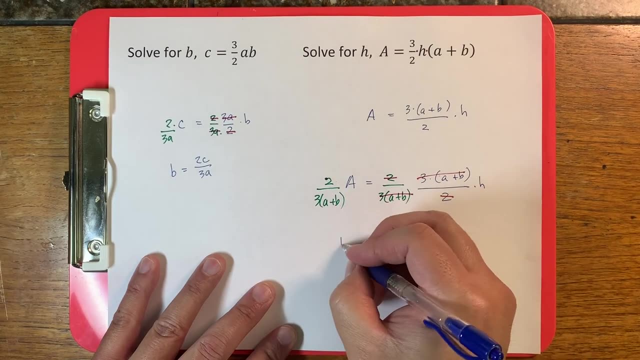 2 over 3 a plus b, And then we're going to cancel this out, cancel this out, cancel that out, cancel that out. And then we get: h is equal to 2a divided by 3 a plus b, And I think that's a perfectly fine answer. 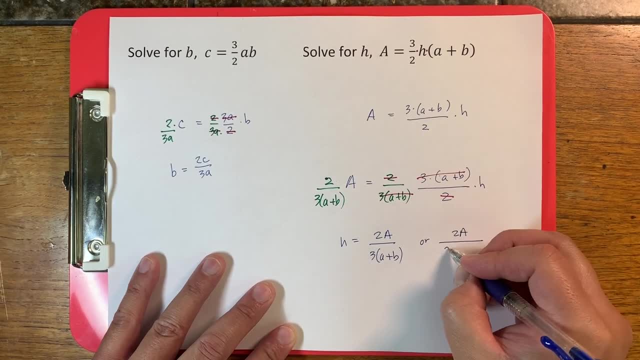 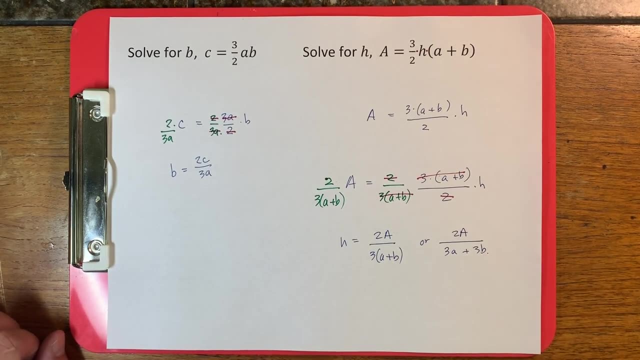 But some people will feel pressured or nervous and they'll distribute, And that's a perfectly fine answer. also Now, if this video helped you, please like and subscribe so other people can find it. Thank you.